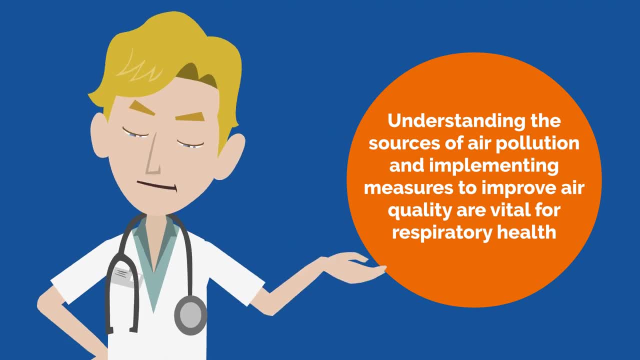 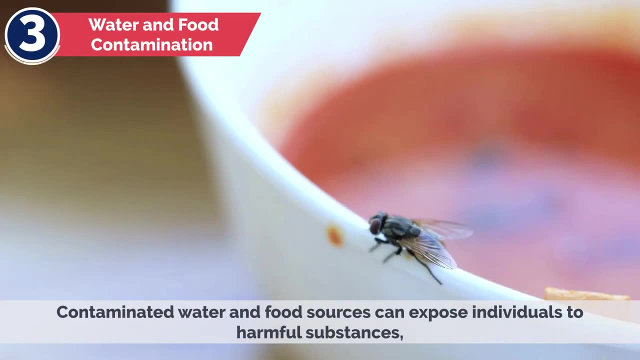 Understanding the sources of air pollution and implementing measures to improve air quality are vital for respiratory health. Segment 3. Water and Food Processing. Segment 3. Water and Food Processing. Segment 3. Water and Food Processing. Contaminated water and food sources can expose individuals to harmful substances, leading to gastrointestinal issues, infections and long-term health problems. 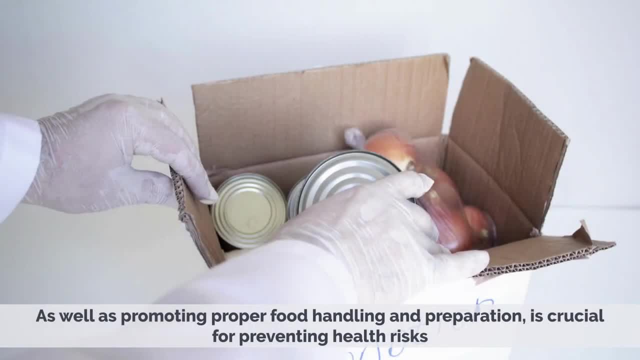 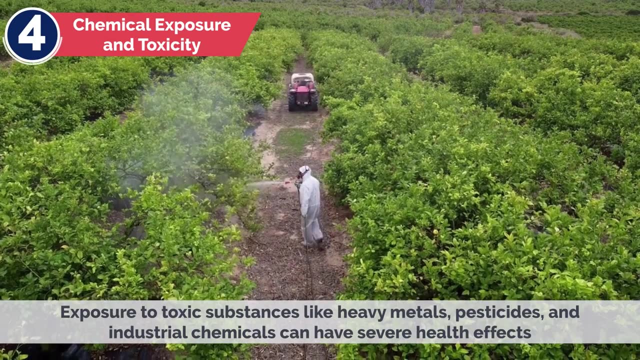 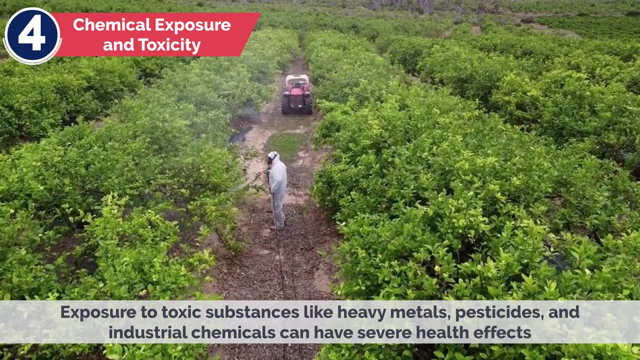 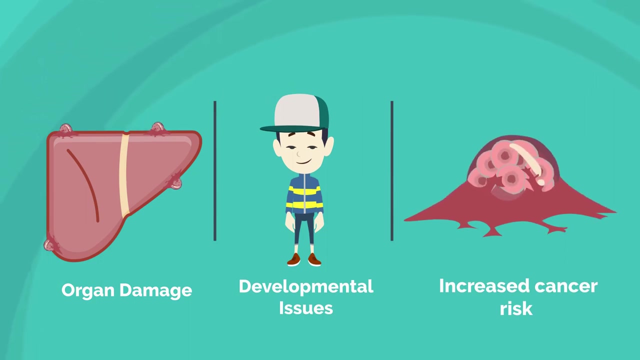 Ensuring access to clean and safe drinking water, as well as promoting proper food handling and preparation, is crucial for preventing health risks. Segment 4. Chemical Exposure and Toxicity. Exposure to toxic substances like heavy metals, pesticides and industrial chemicals can have severe health effects, including organ damage, developmental issues and increased cancer risk. 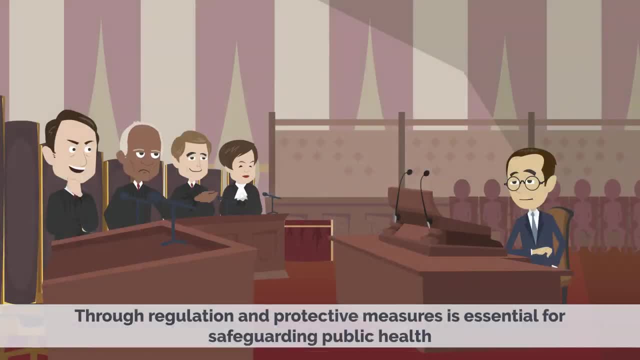 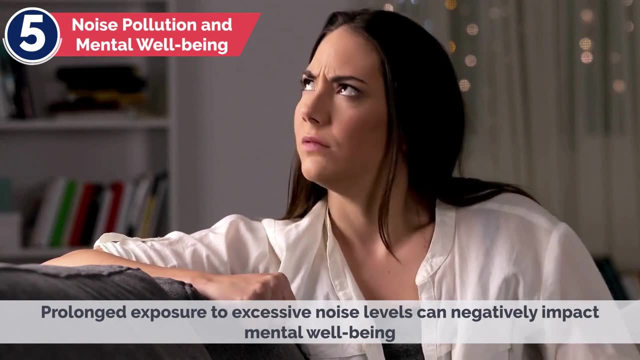 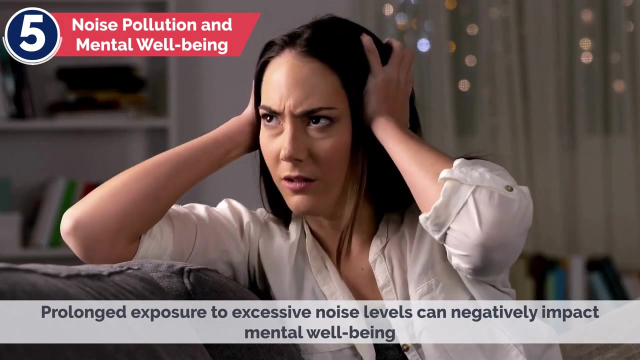 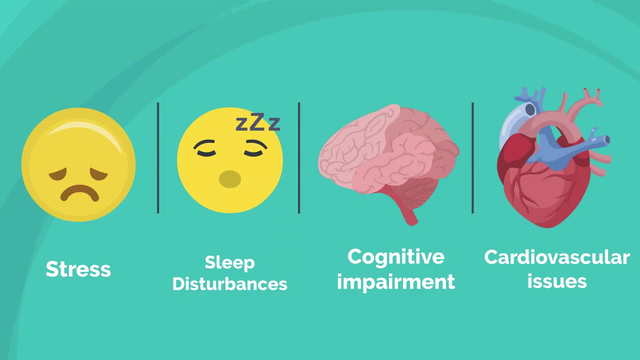 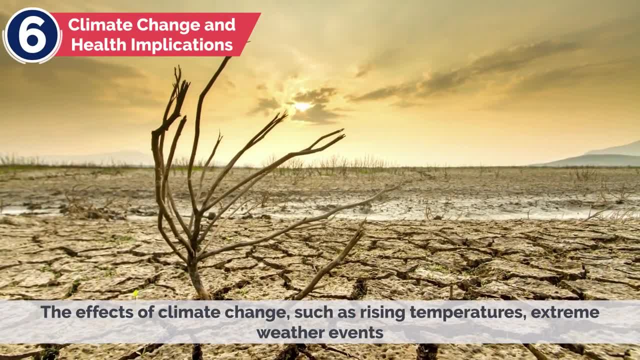 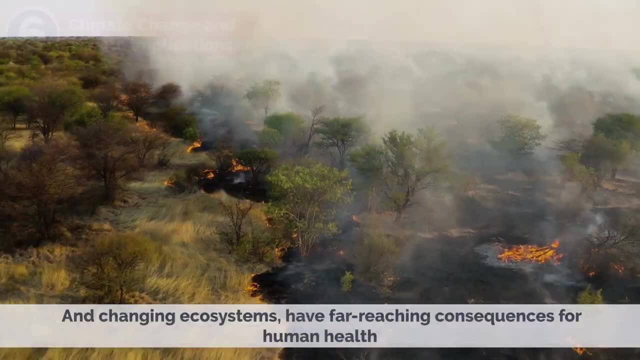 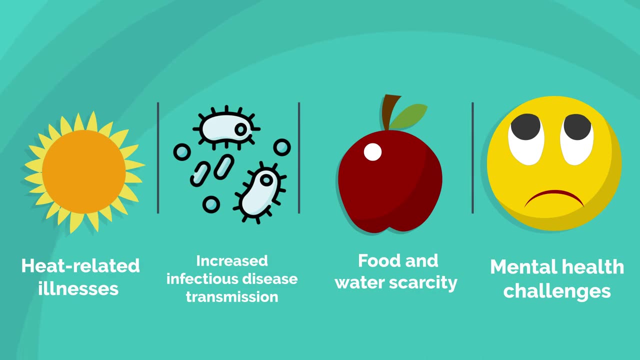 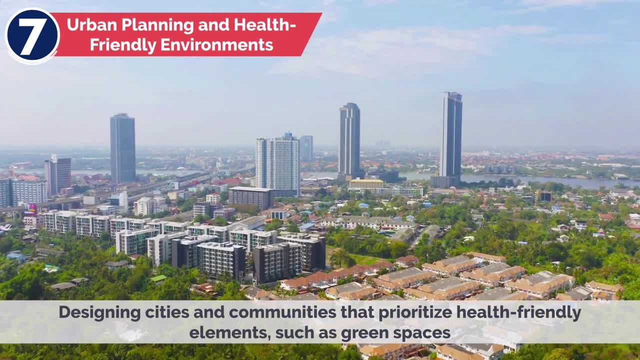 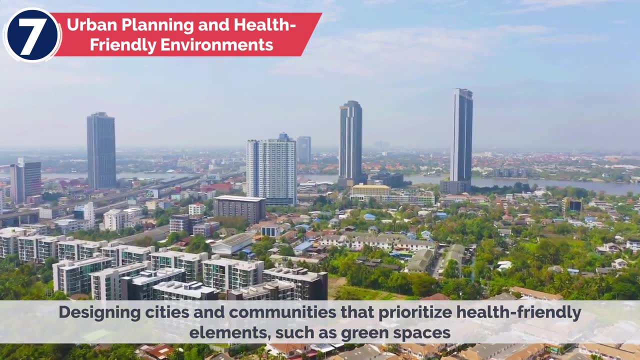 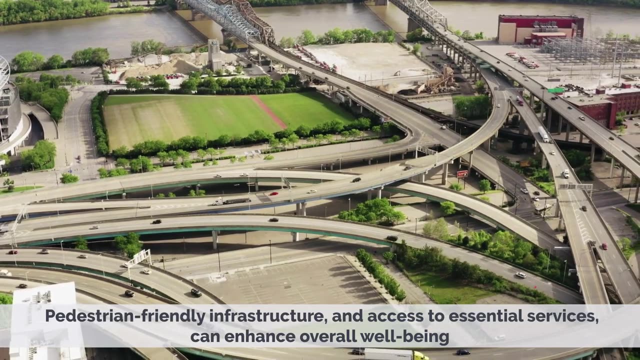 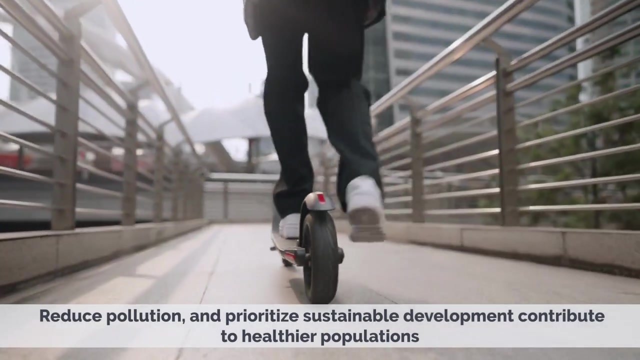 Segment 7. Urban Planning and Health-Friendly Environments. Designing cities and communities that prioritize health-friendly elements such as green spaces, pedestrian-friendly infrastructure and access to essential services can enhance overall well-being. Urban planning strategies that promote active lifestyles, reduce pollution and prioritize sustainable development contribute to healthier 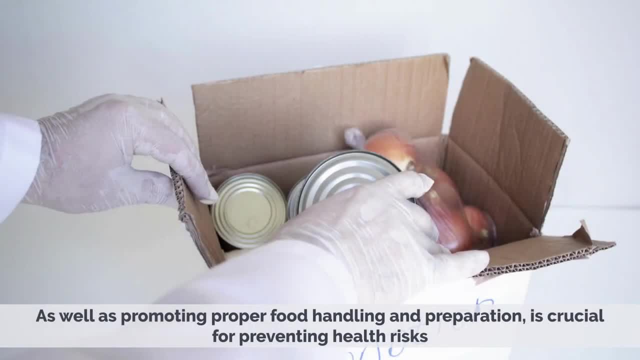 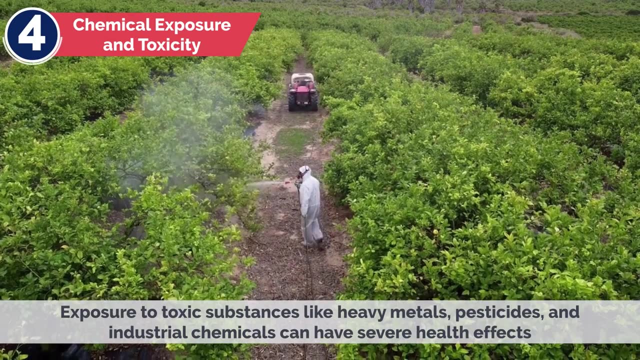 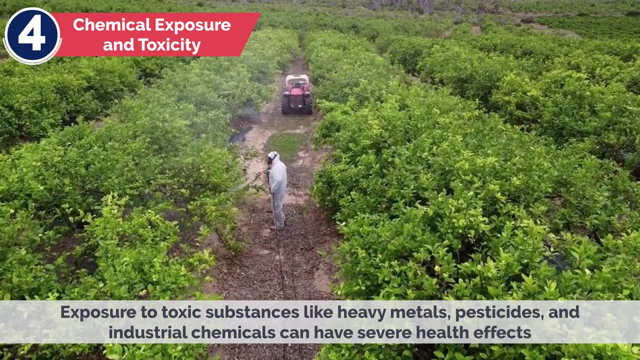 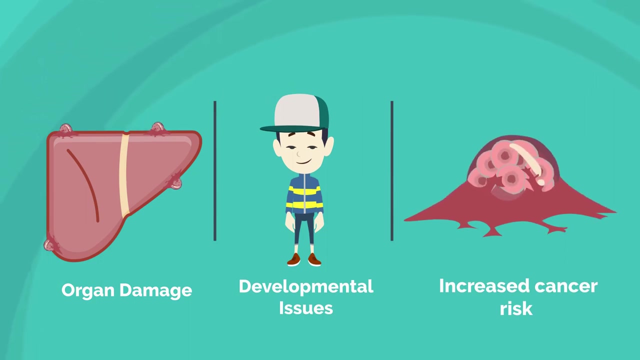 Ensuring access to clean and safe drinking water, as well as promoting proper food handling and preparation, is crucial for preventing health risks. Segment 4. Chemical Exposure and Toxicity. Exposure to toxic substances like heavy metals, pesticides and industrial chemicals can have severe health effects, including organ damage, developmental issues and increased cancer risk. 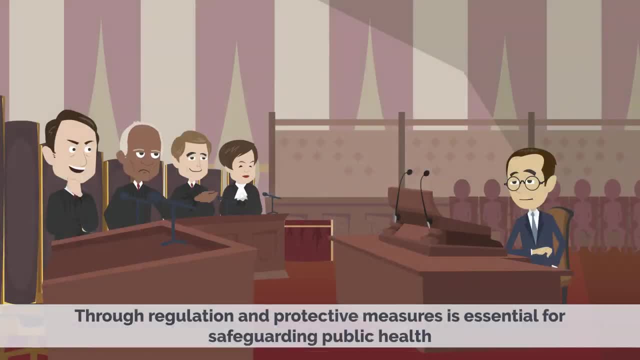 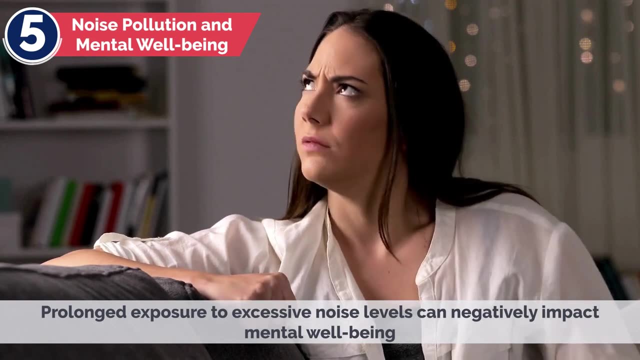 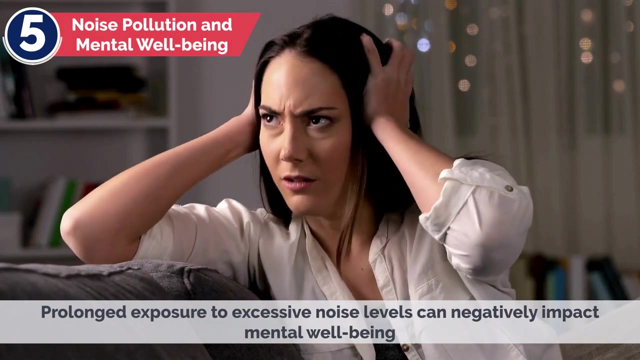 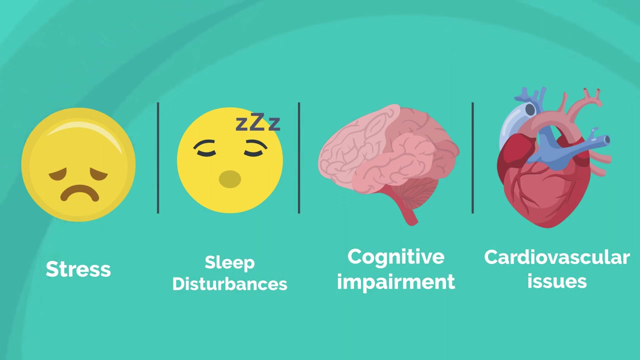 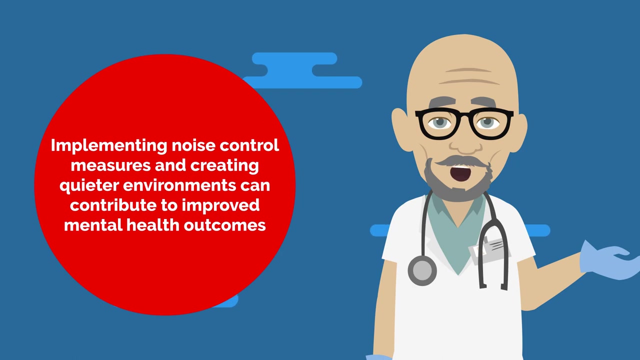 Identifying and minimizing exposure to hazardous substances through regulation and protective measures is essential for safeguarding public health. Segment 5. Noise, Pollution and Mental Well-Being. Segment 5. Noise Pollution and Mental Well-Being. Implementing noise control measures and creating quieter environments can contribute to improved mental health outcomes. 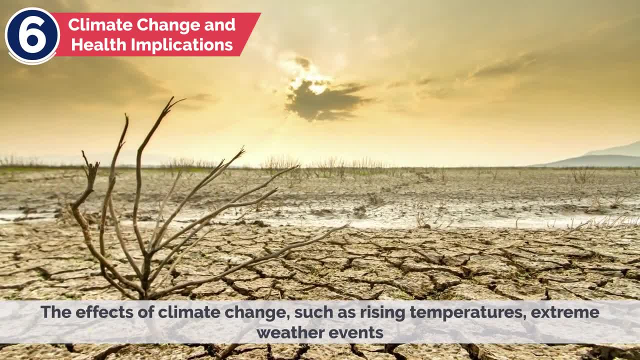 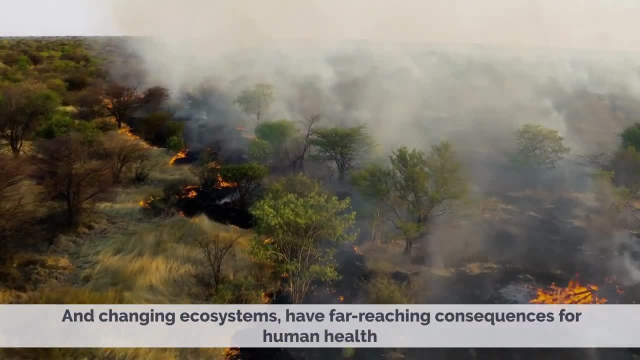 Segment 6. Climate Change and Health Implications. Segment 6. Climate Change and Health Implications. The effects of climate change, such as rising temperatures, extreme weather events and changing ecosystems, have far reaching consequences for human health. The effects of climate change, such as rising temperatures, extreme weather events and changing ecosystems, have far reaching consequences for human health. Segment 8.. Manifest point-of- profit Providenced health. STAR® 750973,. Amitda�Ht383204,. 은�Therapy Share mom and daughter. create breacak hires in the US. president blue intern: Sarah Johnster. 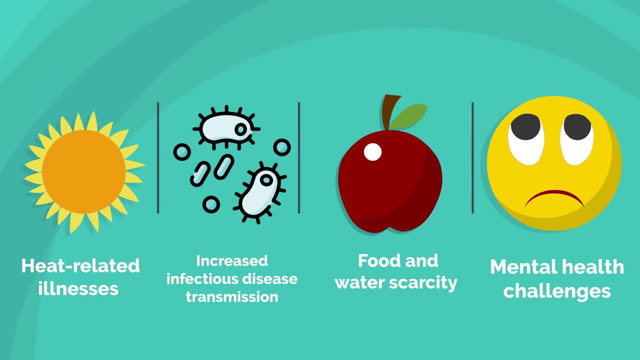 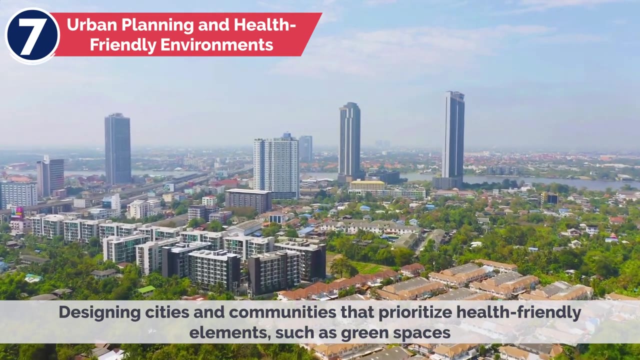 Climate-related health risks include heat-related illnesses, increased infectious disease transmission, food and water scarcity and mental health challenges. Segment 7 – Urban Planning and Health-Friendly Environments: Designing cities and communities that prioritize health-friendly elements such as green spaces. 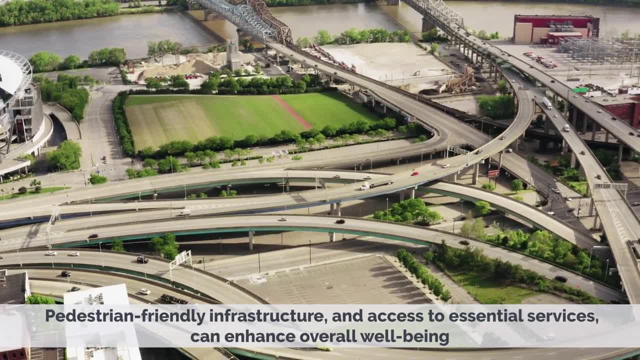 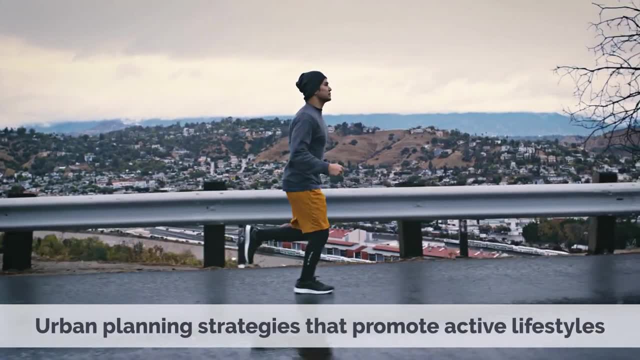 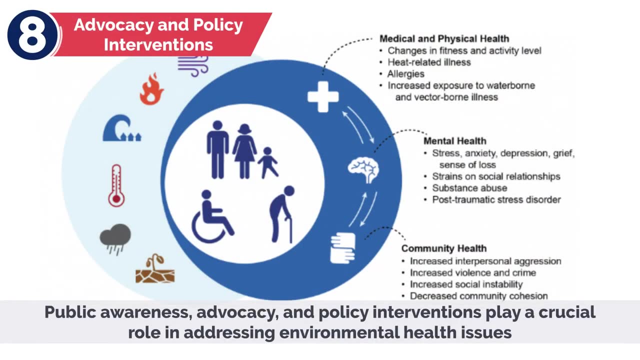 pedestrian-friendly infrastructure and access to essential services can enhance overall well-being. Urban planning strategies that promote active lifestyles, reduce pollution and prioritize sustainable development contribute to healthier populations. Segment 8 – Advocacy and Policy Interventions. Public awareness, advocacy and policy interventions play a crucial role in addressing environmental health issues. 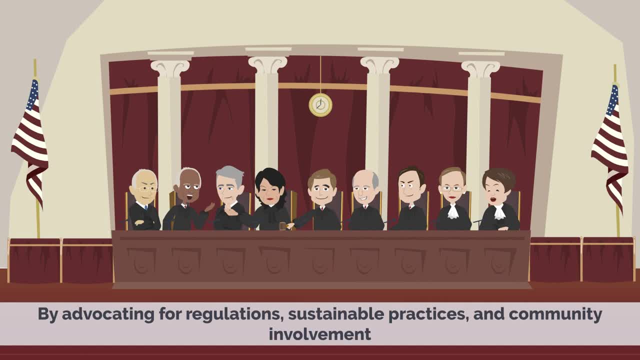 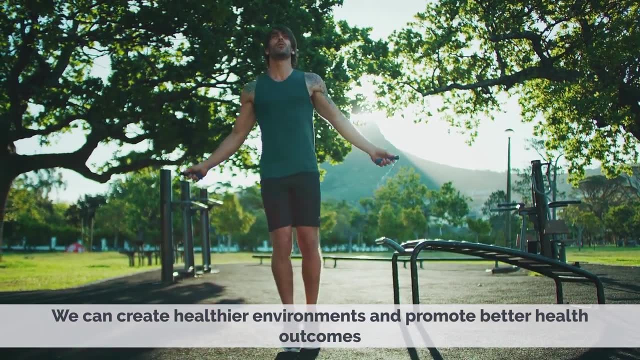 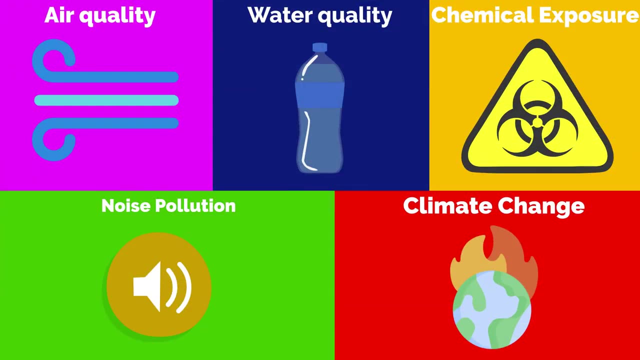 By advocating for regulations, sustainable practices and community involvement, we can create healthier environments and promote better health outcomes. The impact of environmental factors on our health is profound and wide-ranging, From air and water quality to chemical exposure, noise pollution and climate change.